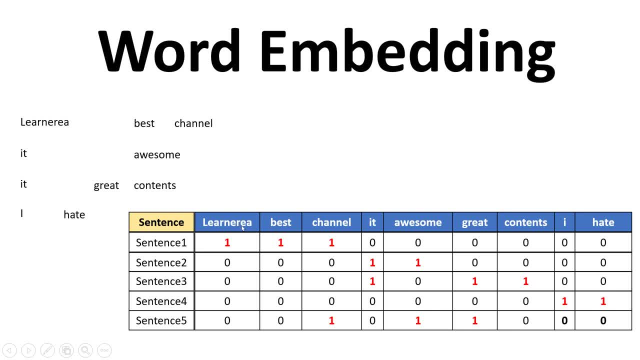 this Right. So if you see over here, it has extracted all the features from this applied data and then it is doing the, you know, representation of the text in form of number. So this is this could be. this could be an example of one hot. 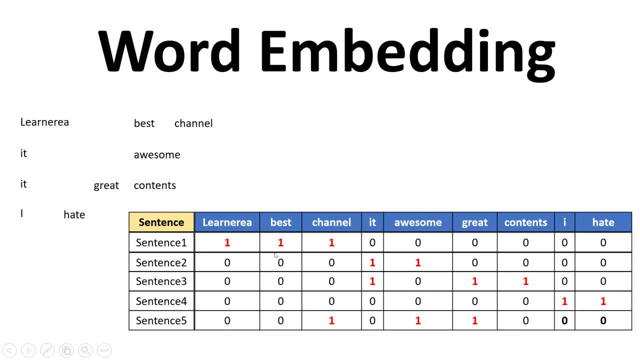 encoding. Similar thing happens in bag of words also, But numbers gets repeated in bag of words. I mean, it will be more than one if the particular word gets repeated into the sentence, Right? So this is it. This is word embedding in a nutshell. Now there are multiple ways of word. 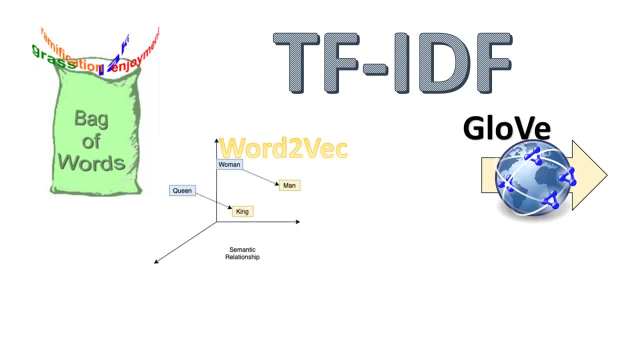 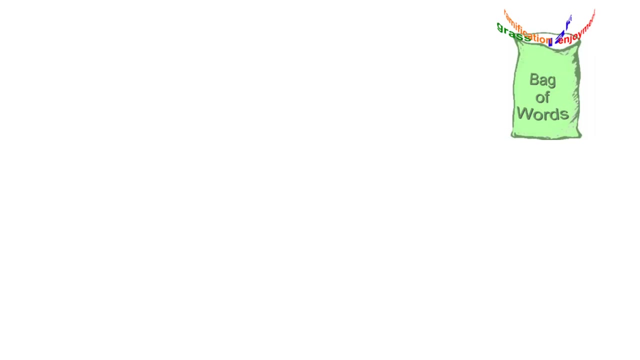 embedding, For example, bag of words TFIDF, WordVec, Glove and BERT Out of this bag of word IDF we have already covered. right link is given in the description section. You can just check that out. However, I'll just try to give a brief about it. So in bag. 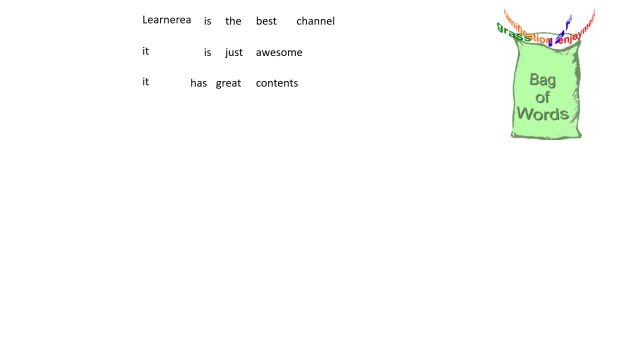 of word. what we do is: this is the sentence which have been supplied. For example, you do some sort of please pre-processing and then it extracts the list of features and prepares vocabulary list. Then it will put these sentences and it will do the encoding. 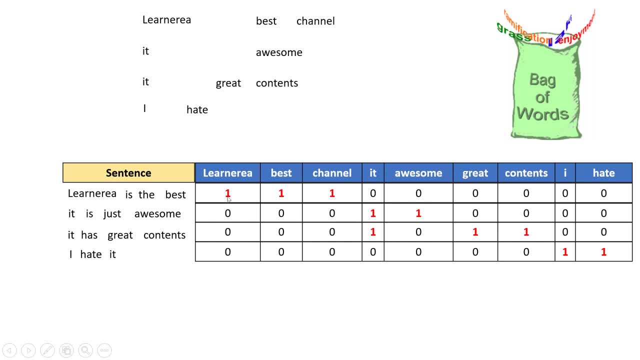 something like this: Wherever it finds a matching word in the given dla for this line, you can install this line, the given sentence. it will say one. wherever it doesn't finds, it says zero, what i just explained. for example, if a word is repeated in a given sentence, for example, let's say best is repeated. 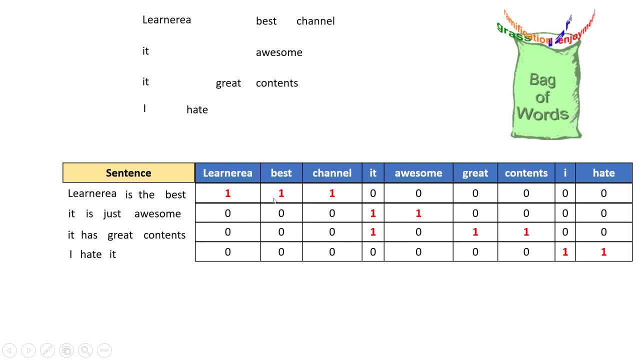 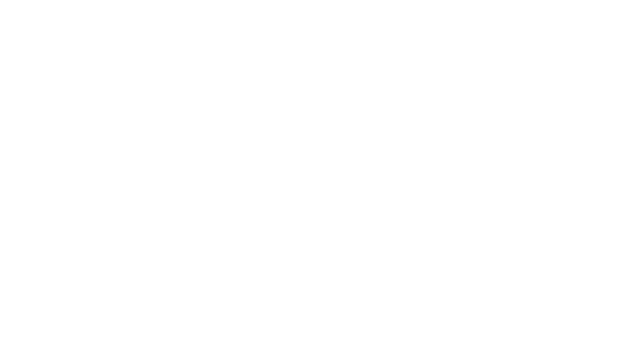 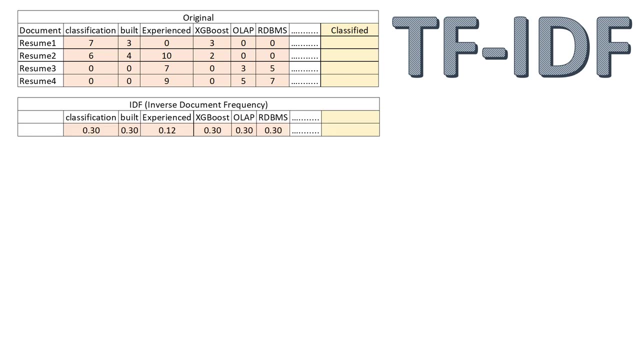 in this particular sentence, then instead of one, it will be two. if it is repeated three times, it will be three, and so on. so this is how back of word works. in tf, idf, what happens is: this is the supplied data, this is the supply data which you would have, and then it will calculate the inverse. 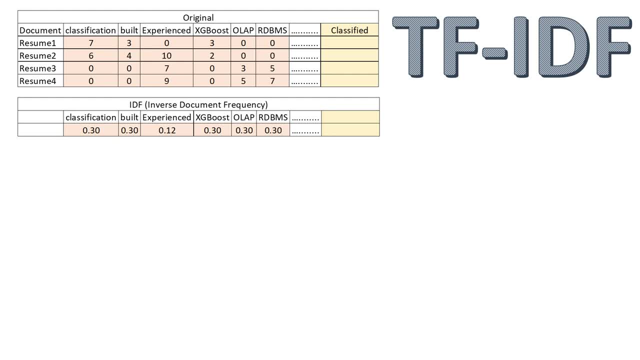 document frequency. now, if you want to understand what inverse document frequency is, i highly recommend. and then the next thing which we need to do is find the term frequency. and after finding the term frequency, the last thing which we're going to do is multiply both of them and get the 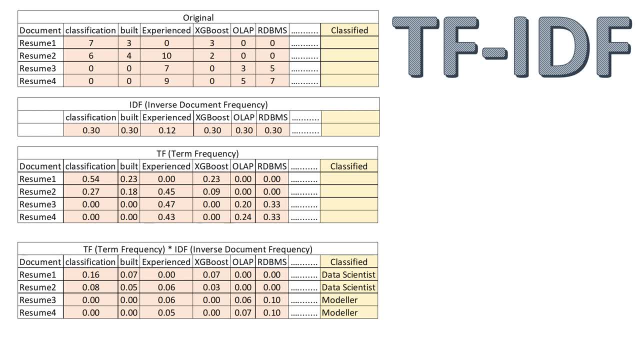 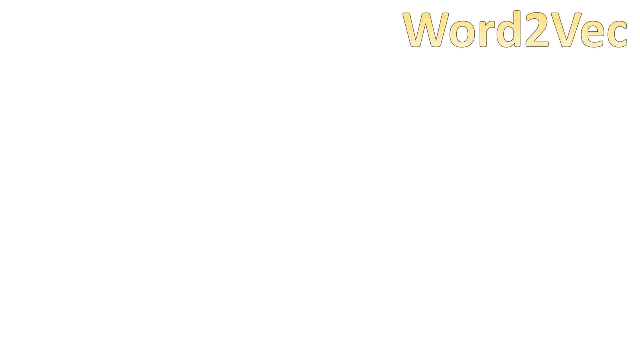 df, idf value. based on that, before that, we can do the prediction or we can build the predictive model. okay, now, this is a very important thing to consider. okay, if you are not familiar with måsik, the main thing which we're going to cover in this video today is word to wake. What word to wake? 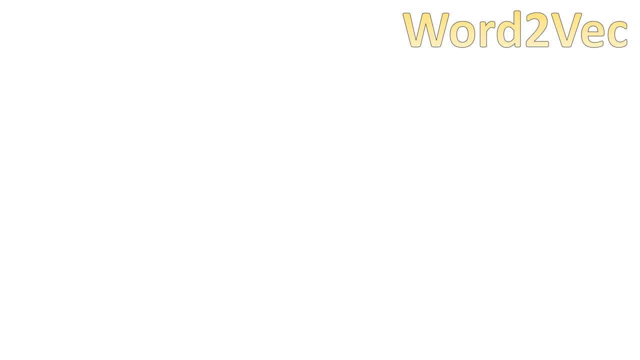 does exactly. This is like I said. this is also one of the word embedding technique and which is very important, simple and important thing, right? So, for example, let's try to understand word to wake with the help of an example. Let's say: you haven't given these two sentences When you make. 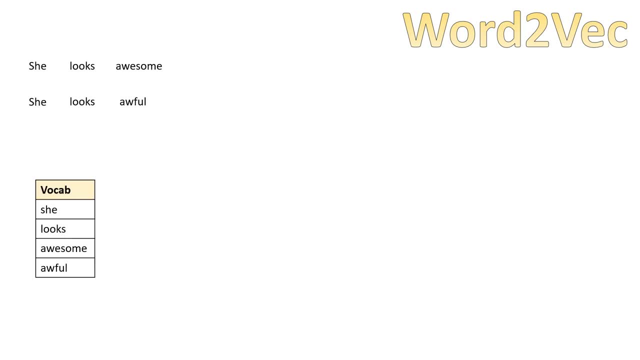 word to wake. what it does is it creates, using the supply data, it creates list of vocabulary and it does some sort of scoring. Now you must be getting how does it does the scoring right? How did it get to know that this 0.01 is for she, 0.02 is looks and negative, 0.05 is awesome, and so on? 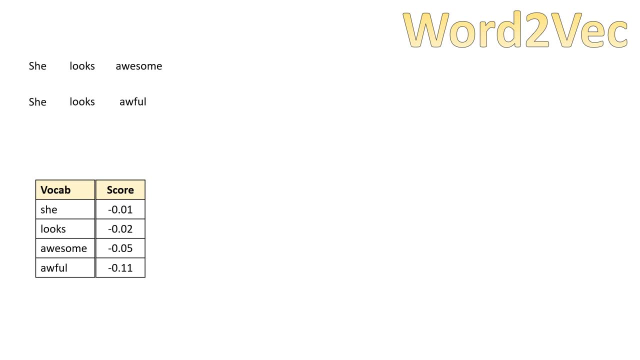 right. So okay, before I proceed further, let me tell you: these scores given over here are completely synthetic. This is not the real score which word to wake has generated, just for the understanding I've given it over here. So now, 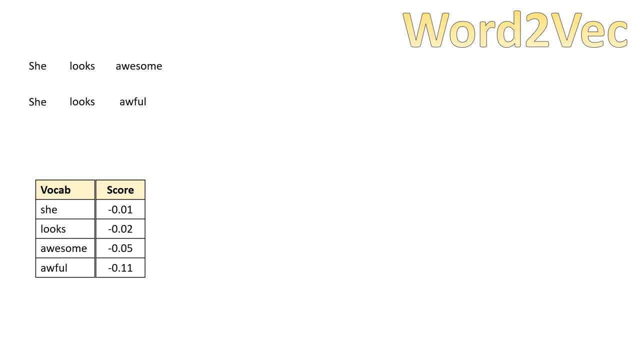 coming back to the point, how it does the scoring. So to make you understand this concept, let me tell you that word to wake is based on two. I can say sub models, right, Which is nothing but CBOW, plus skip gram, right, CBOW is nothing but the continuous bag of words. and skip gram These two. 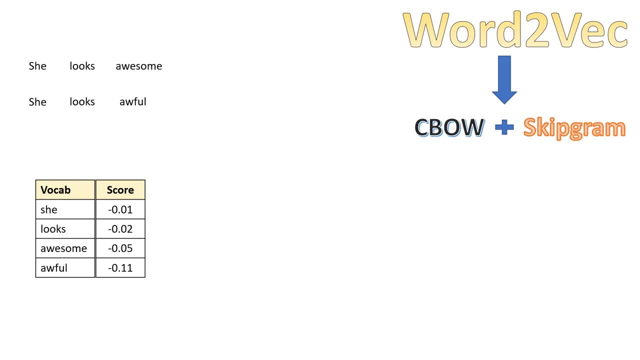 techniques are at the core of word: to wake. What these two techniques are we will see in upcoming videos in detail. Over here, let's understand how these two works. So both of these two techniques works on cosine similarity Based on the cosines. both of these two techniques use cosine similarity. 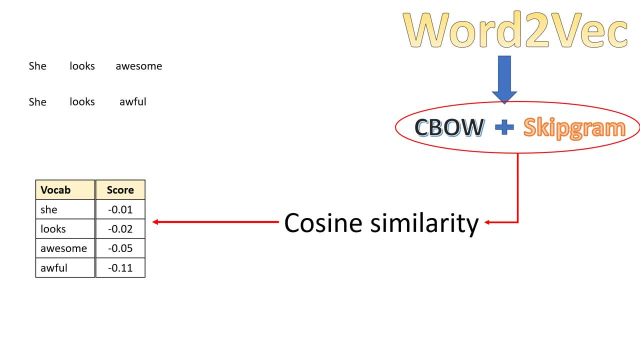 and does this kind of scoring. Now, what cosine similarity is? we are not going to get into the mathematics in this video, at least In upcoming videos. if you are interested, I will cover that. Now let's understand the scoring in non-mathematical. 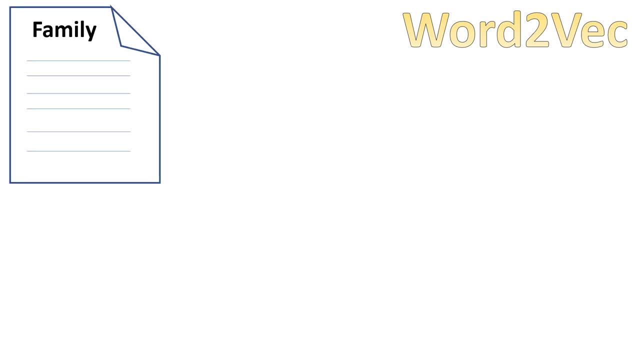 way. For example, here you have a document which is about a story of a family And this is, let's say, this is a piece of information you know, fetched from this document, just to show you right, Nothing else, right? This is just to take a reference. So let's say, the whole document is: 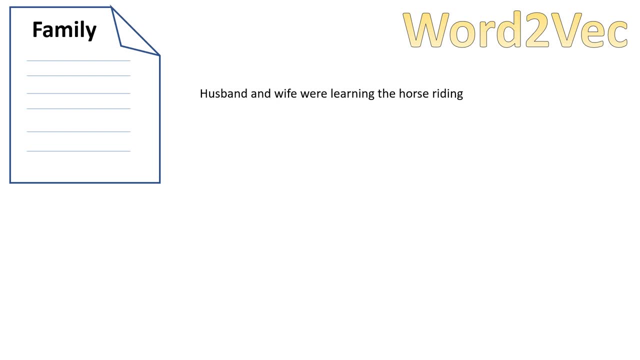 applied to word to wake model The training. So what it will do is it fetches the document and prepares a list of vocabulary right, Prepares a vocabulary list right And then inside this it will create invisible set of properties, Or maybe you can do say features also. This is something which you 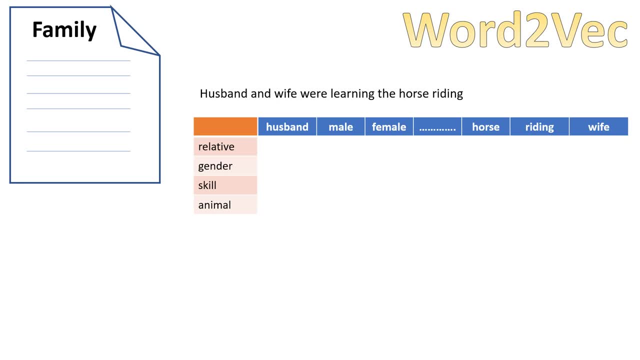 want to be able to see And basis on this, it will do the scoring, For example, relative gender, scale and animal. These are the inbuilt properties of these words, right, You can say? or the feature of these words. So wherever it matches to the word, it will produce the it will. 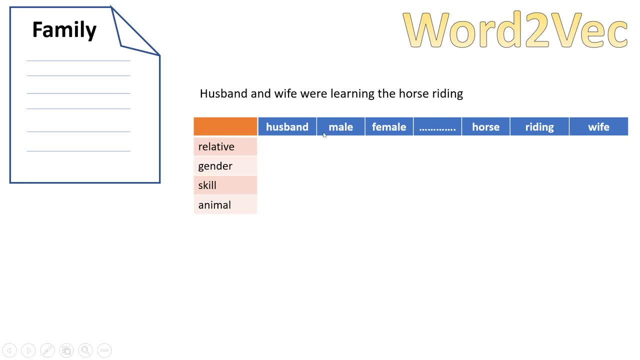 produce some sort of you know- scoring. And it also, like I said, it works on CBOW, which is nothing but continuous bag of words. Continuous bag of words takes the input and you know, take multiple input. It takes one output, right And skip gram works in the other way, right? So let's come back to the 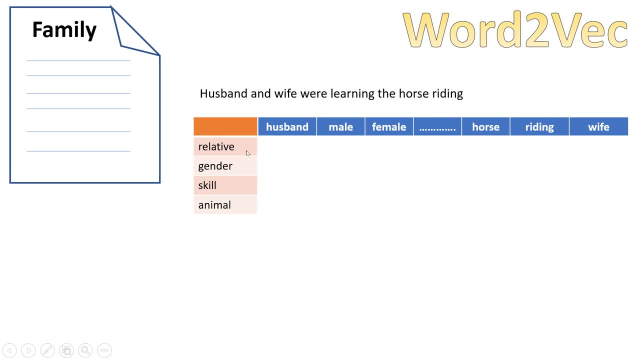 point, And over here you see a husband. Yes, it's a relative. I mean, husband is a relation, So here what you get is value one. Similarly, husband has a gender which is male in nature, So male. 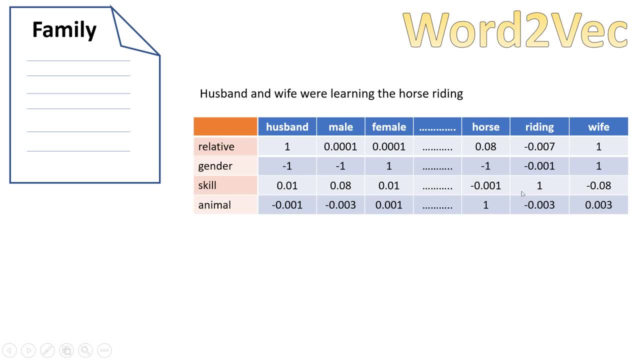 we are representing through minus one. Similarly, we have the score for each of these words. Now, what you see over here is, none of the word has a value Of zero, the way we used to have in bag of words. So that's the other advantage. Now, this is how. 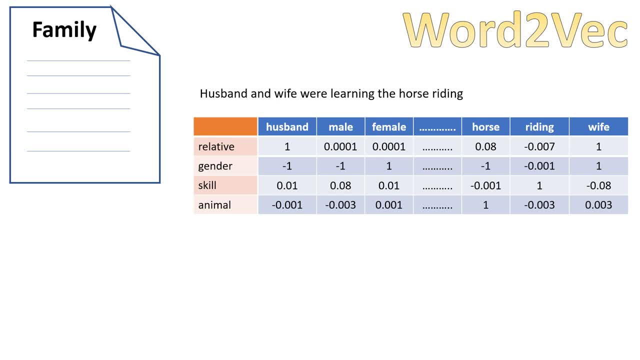 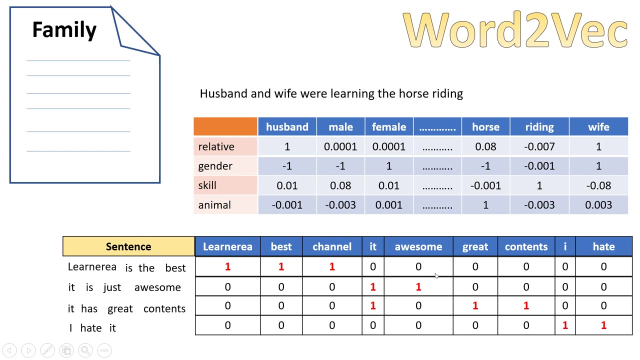 you can. I mean, this is how it does the scoring. Now, what is the advantage of having this? Okay, What is the advantage of having this? We will see that first advantage is, which I just covered, like in the bag of words, we saw that wherever it doesn't match to a word, it produces zero for. 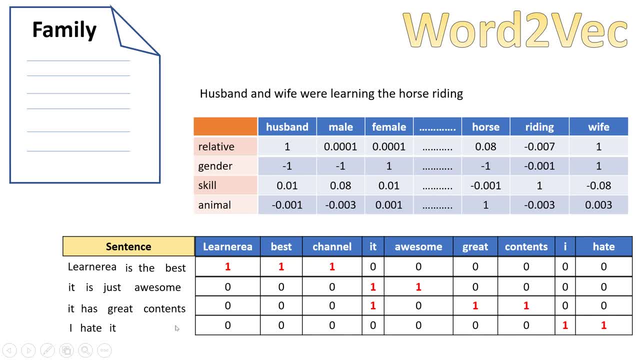 that And that's how, when you keep on adding the sentences, it will keep on adding another features and it will keep on producing zero wherever it doesn't find a match right, Which results in a sparse matrix. That's called the sparse matrix. What is the other advantage of it? That's really interesting.